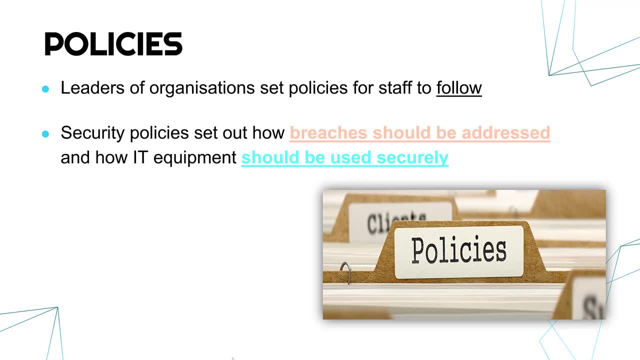 should be used securely. so how should the staff be using the computers to lessen the risk of an attack? now, it's really, really important, I would say, that staff are trained in how to follow the policies. if you ever get an exam question on, you know what should a company do to improve their 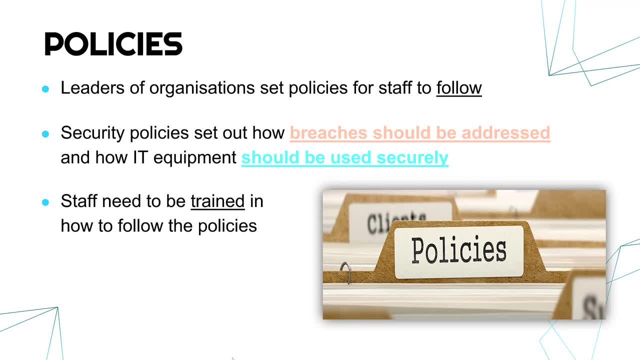 security. I would always write about training, because staff make mistakes. people don't always know how to be safe online. they make silly accidents. they need training. it's not just enough to read a long document. they need to be trained on how to enact these policies, and often from a kind 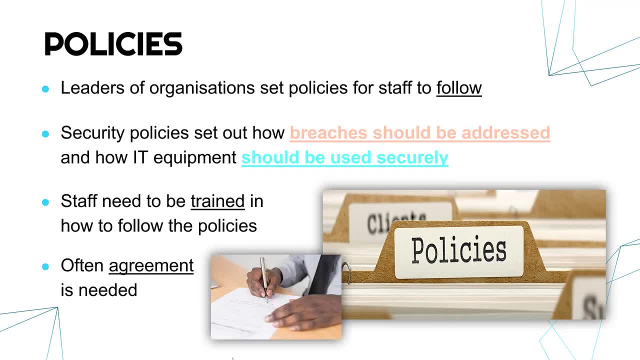 of company's perspective. it's not just about training, but it's also about training and it's really important to be trained on how to enact these policies, and often from a kind of company's perspective, for a sort of legal perspective. often you'll be asked to sign a policy to show. 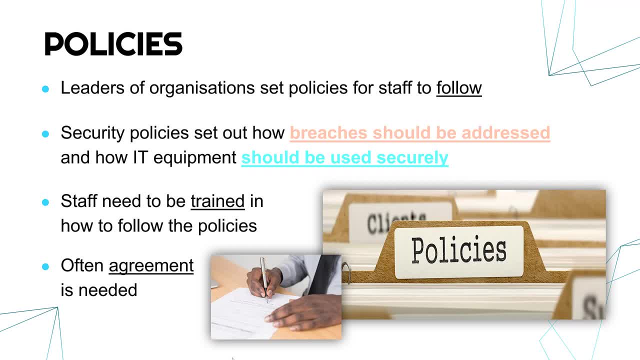 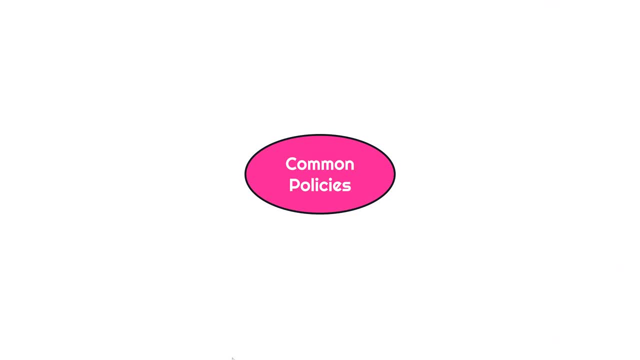 that you agree to it. now there are loads of policies, of course, a lot unrelated to IT, but some of the ones which are common and are connected to security are these, starting with a policy about staff access rights. so this policy will most likely set out who should be able to view. 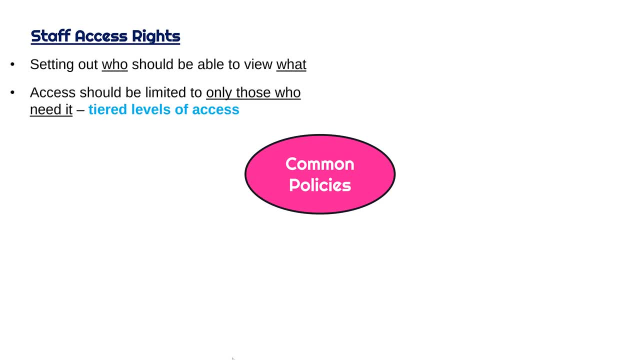 what? so the idea is, the principle is, access should only be given, should only be limited to only those who need it. so you know, everybody in an organization should not have the same level of access. so the principle that you have these different levels of access is called tiered levels of access. the CEO should possibly have access to all of the data. 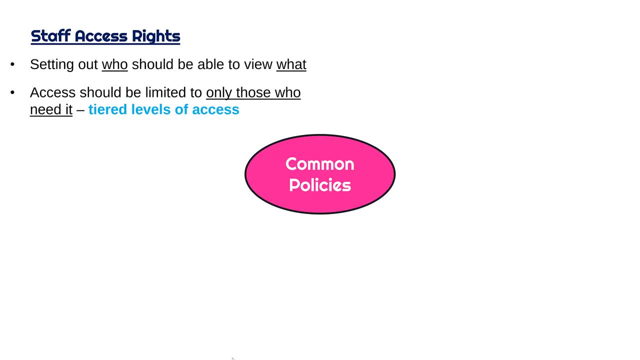 in the company, but a junior member of staff should maybe only have access to a very, very small amount. it's silly giving access unnecessarily because it's just opening the risk of mistakes getting made and somebody stealing or changing the data. so this staff access rights policy might set out who should be able to access what. 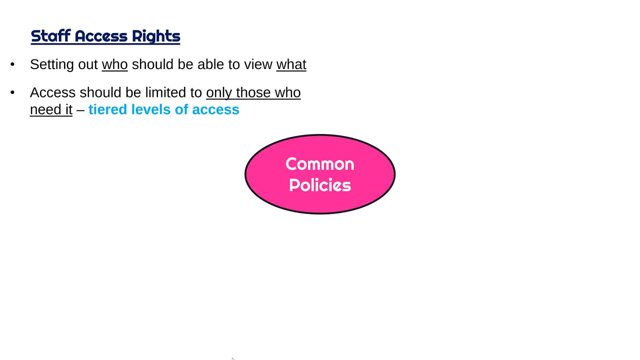 and maybe the consequences for somebody breaking these rules. another kind of category of policy which may be put into something called an acceptable use policy. it's just about the different responsibilities staff have. so this is, for us, in particular, focusing on the expectations on the staff- staff for how they should be using the IT securely, so setting out what they should be doing and why. 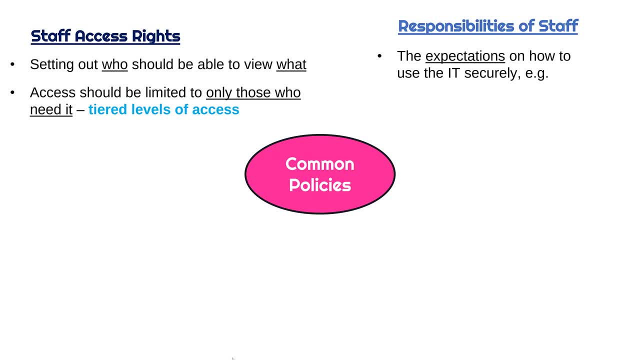 hopefully, in order to make things as safe as possible- hopefully, so. some examples might be things like: you know the need to set complicated passwords, and the policy should say what they mean by a complex password. another policy might be to encrypt your personal data, and again, the policy should say how exactly you would do that. maybe you are told to not write login details down. 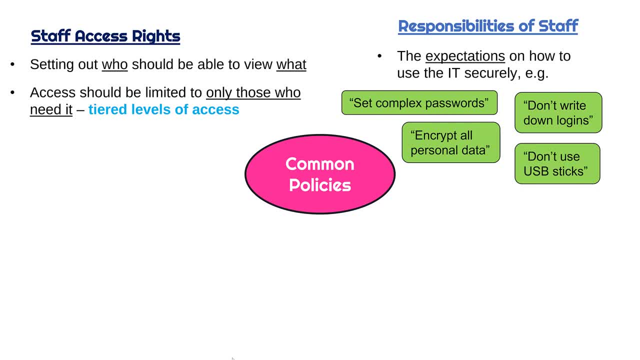 and it should say why that's important, and maybe it will say you can't use USB sticks, the reasoning possibly being because it could be used to introduce malware onto the computers or they can be used to take personal data out of your systems. so that might be part of a policy. 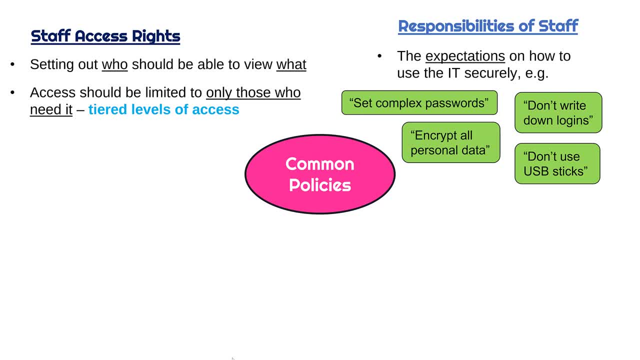 these principles will vary between different organizations. another policy or group of documents which may get made are risk assessments. so risk assessments are these often quite long, assessing the level of risk. okay, so they're trying to put a number, most often on how likely a risk is to occur and what impact would there be if the risk actually happened in terms of a policy. 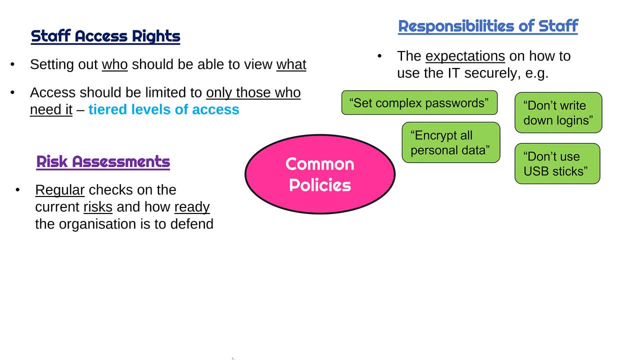 what the policy might be that you need to have regular checks on the current risks and also checking how ready the organization is to defend against these risks. if every two years you have a check on the risks, that is obviously not a great idea because every single day 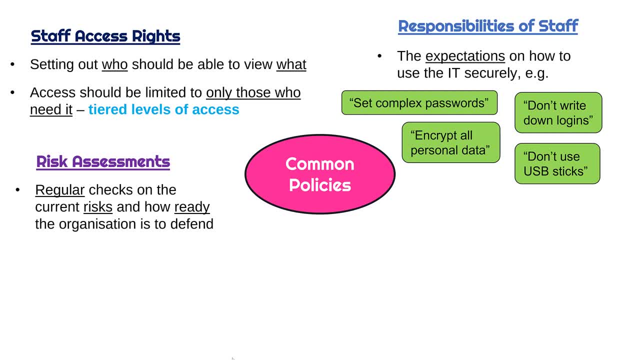 there are new attacks, whereas if you do a risk assessment every month, that's much more suitable because you know things don't change that much month to month. maybe now in terms of what this document looks like: I've shown you this picture before in a previous video about. 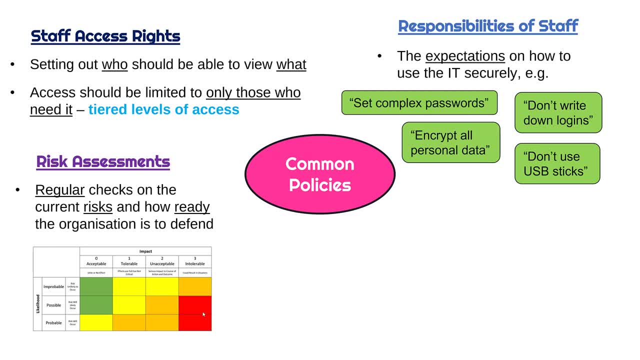 risk, but often there'll be sort of colors or numbers assigned to the level of risk. high risk means that it's going to cause lots of issues, it's going to have a big impact, but also it's going to be quite likely and over time the risks shift around. one thing which i'll 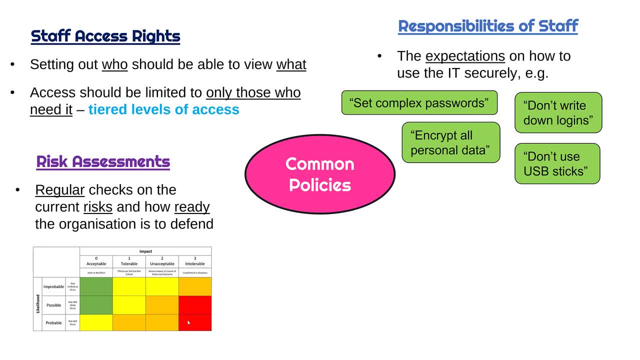 might be relatively minor in one year, the next year might be deemed a much higher risk because it's much more common. for example, ransomware 10 years ago was not nearly as big of a problem. in the last few years, ransomware has become a huge issue for companies, and so over time the 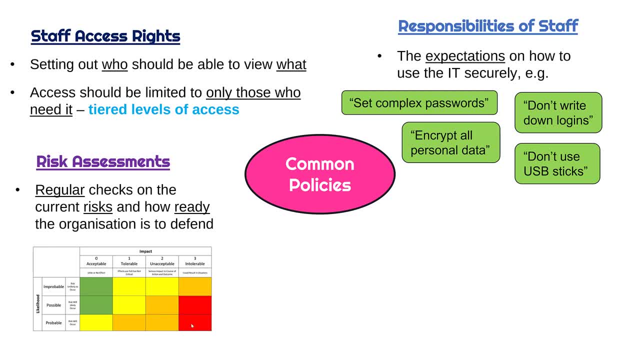 risk assessment changes and it updates this risk. so, as a policy, it's all about doing this often and being aware of the risks and how they might change. linked to this will be assessing the effectiveness of your protection measures. so these protection measures are for things which are trying to keep you safe and, over time, you should be reviewing these. do they work, are they? 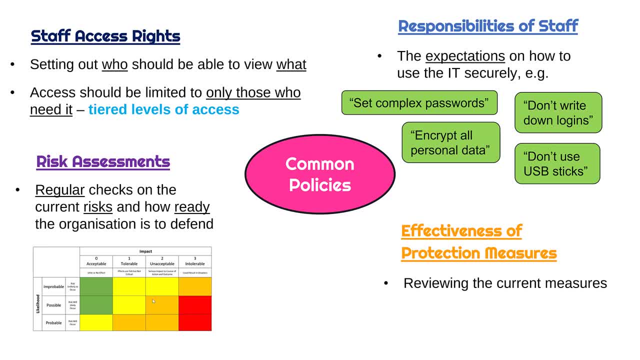 currently effective. as the risks change, do you need to change your prevention measures potentially, and this particular policy may set out things like when and how the current measures are to be tested. sometimes you might employ a, a white hat hacker who is coming in to hack your company. 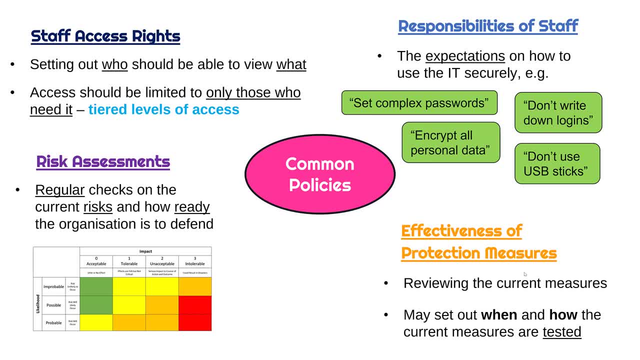 but only to test if your protection measures are working or not. so this policy might set out how that process is going to work, who is going to get used and how that testing is going to get done, a bit like with risk assessments. if you only do this review every couple of years, well things. 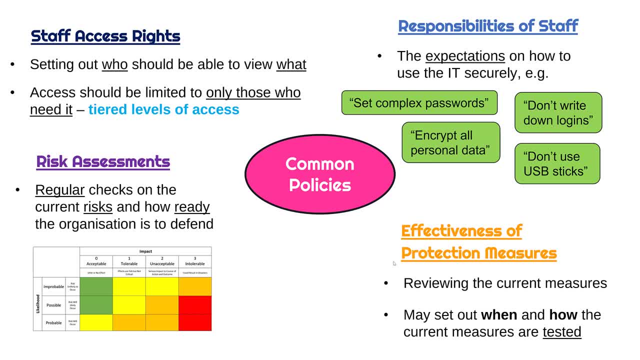 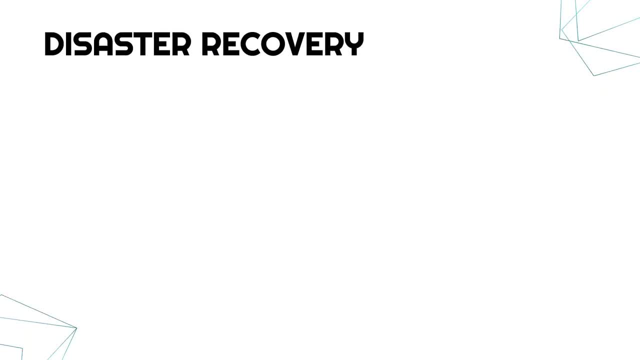 might get out of date very quickly. you know, things change over time. it's important to stay as current as possible. the final policy i want to talk about is a big one, and so i'm giving it its own slide here. the first policy is a security policy. now this policy is setting out what steps are needed. 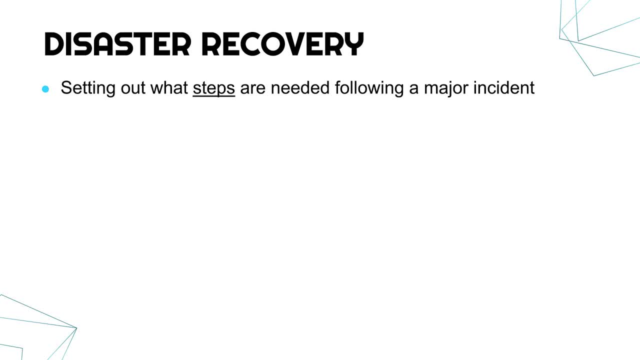 following a major incident. that is what a disaster is: a major problem, a major incident- and we're most often thinking about security. you know you are being hacked. you've got a malware attack happening, you've got a ddos happening, but it can also be accidental things which are unrelated to security. 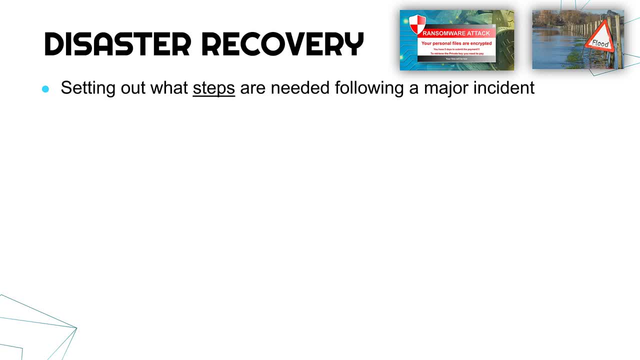 things like a fire, things like a flood- they're not always accidental, but things which are not related security itself. so this policy will set out the steps and it should include the following things, at a minimum, i would say it needs to set out who is responsible for what. who is going to lead on. 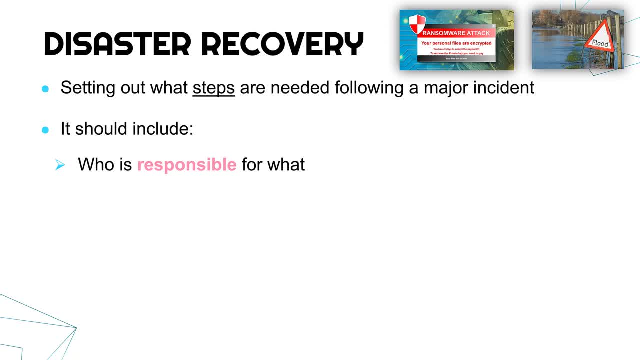 this disaster recovery. who does what job should also say do's and don'ts. so what should the staff be doing? what shouldn't the staff be doing? so, for example, a do might be the staff should back up their data. i don't. should be. maybe don't talk to the media.